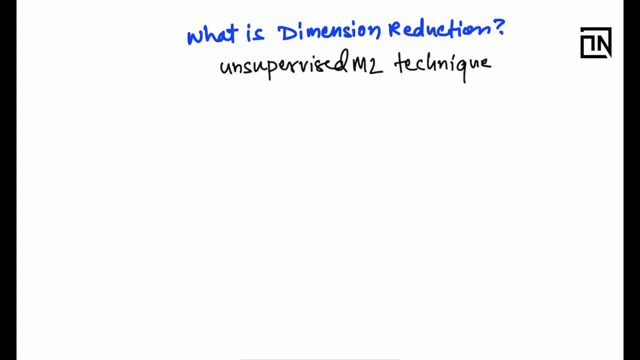 machine learning technique. This technique helps us to reduce large number of columns into small number of columns. For example, let's say you have a data set which you processed explode And finally, after doing all the correlation analysis and converting into dummy variables, you reached at this level where you have one target variable and there are multiple. 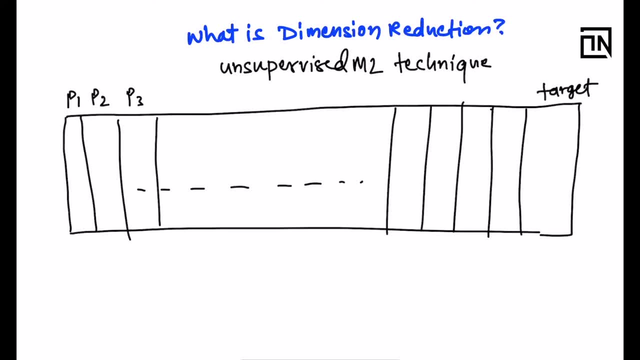 predictors: predictor one, predictor two, predictor three, so on and so forth till predictor 500. So there are 500 columns in your data and one target variable. But hold on, you just said that it is an unsupervised machine learning technique. So let's get started. So let's get started, So let's get. 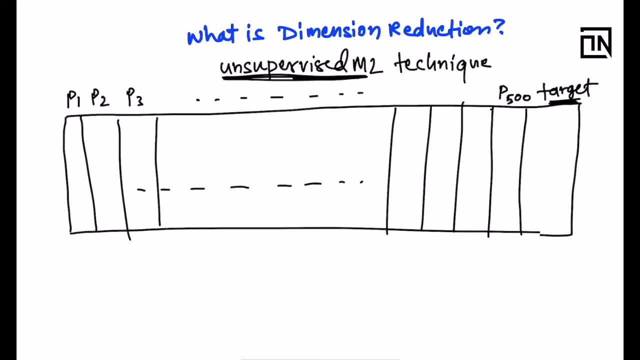 started. You just said that I'm going to introduce an unsupervised machine learning technique to your class, And while we're doing that, I'm also going to explain some rules for how to create the crea용 of data with dimension reduction technique. I. 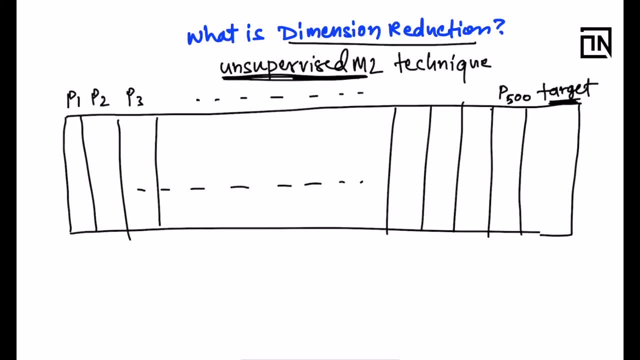 name my class metric бег인. I'll update it in the next lesson because it is my class call day. Oh, so this is it. example one. there you go. So we are going to learn how to create the data all these way down to the sick detail, And for that we need to use. first we're going to take 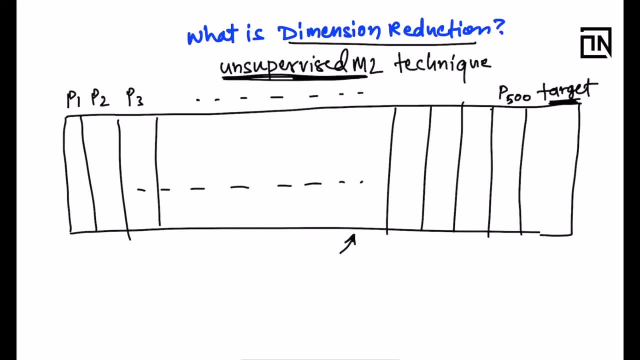 out the stuff into the table, the information that has been stored in the table that we took out and then we're going to do theanki won't show theaja in the video. Okay, and remember we are already working on this in the video, Okay, so, for example, is this stack here And here? 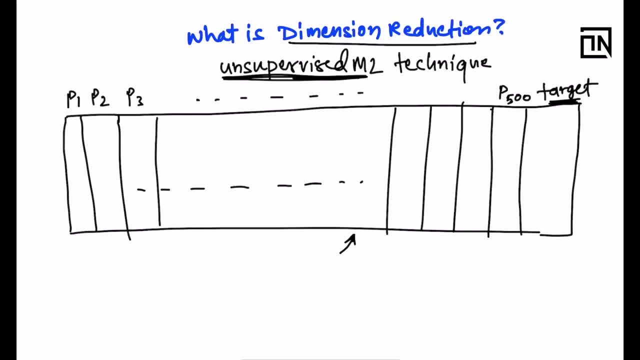 When you take 500 columns into account, this kind of data or more, let's say you have thousand columns or 2000 columns. These kinds of scenarios are very common in text mining. So whenever you are doing natural language processing, you are trying to create a model. 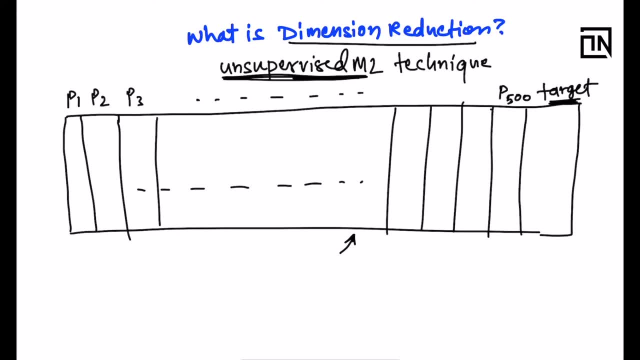 let's say for ticket classification. So the ticket description data needs to be converted into numeric form and then each word will represent one column, also known as the document term matrix In such kind of data sets, thousand columns or 2000 columns of predictors is very common. 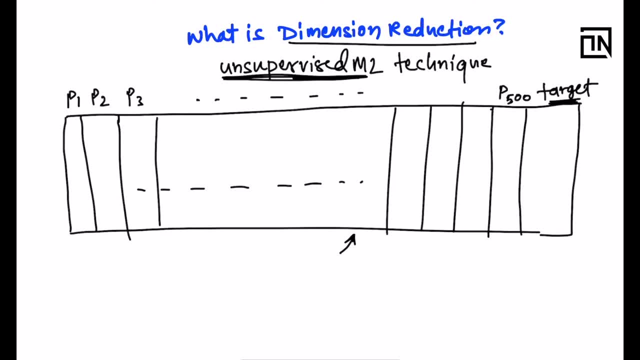 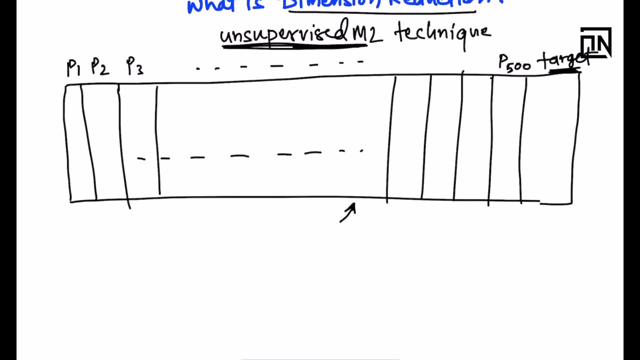 So in such scenarios, let's say, if you use that data to try to fit through a machine learning algorithm, it will take large amount of time and it will be painfully slow. So what you can do is, instead of fitting these 500 columns all together, is there a way in? 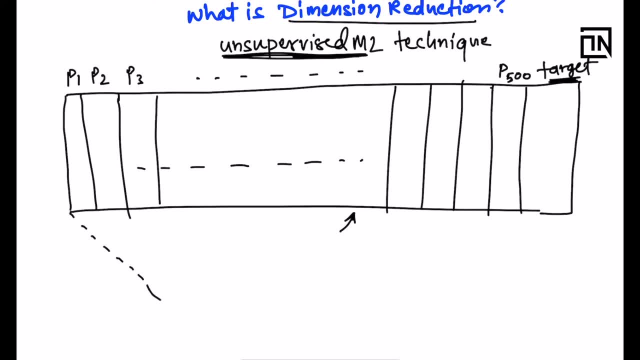 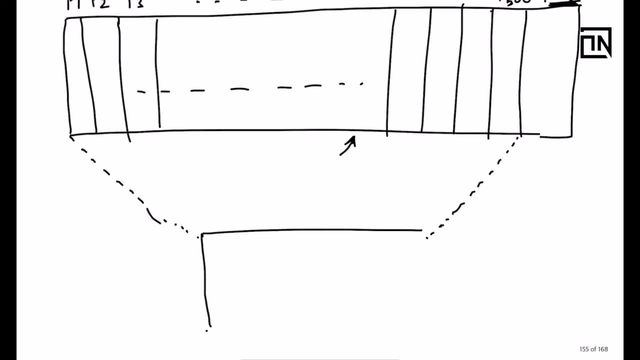 which you can shrink, these 500 columns which you have. So for 500 predictors, I am shrinking the number of predictors only with some smaller number of columns. Let's say, let me call these columns the very famous principal components, let's say principal. 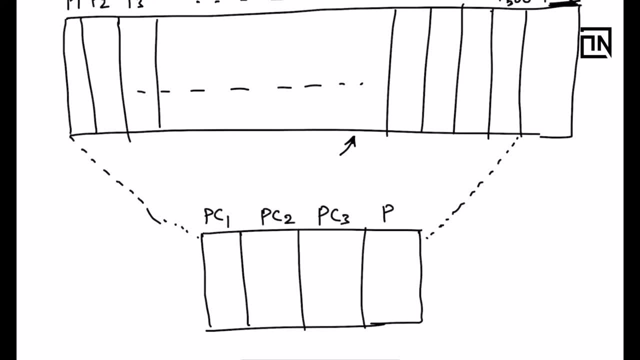 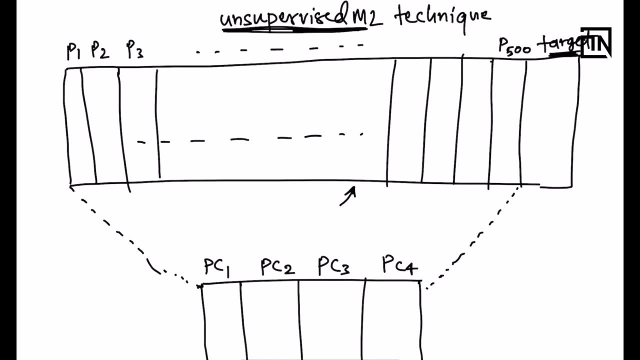 component one, principal component two, principal component three and principal component four. So I am representing these columns, these 500 columns with just four columns, or maybe thousand columns with four columns or five columns. How do we decide these columns? It is based on the algorithm to algorithm. 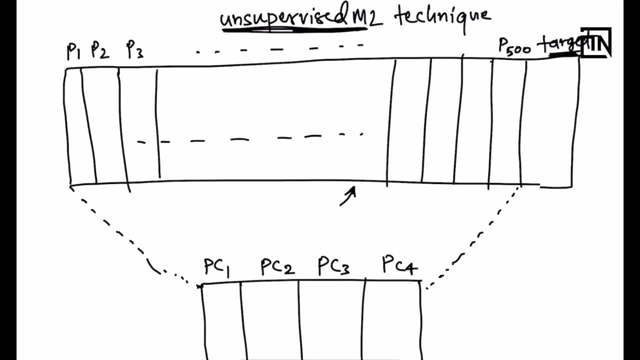 So we will discuss that going further, but this is the overall idea. I am doing some work only on the predictors data, So I'm shrinking the predictors representing large number of predictors with smaller number of predictors. How many predictors should I choose to represent these 500 predictors? 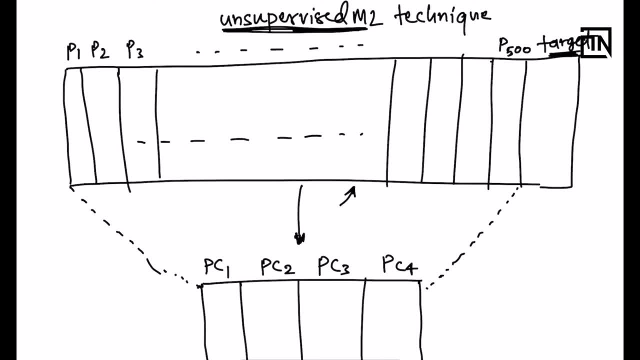 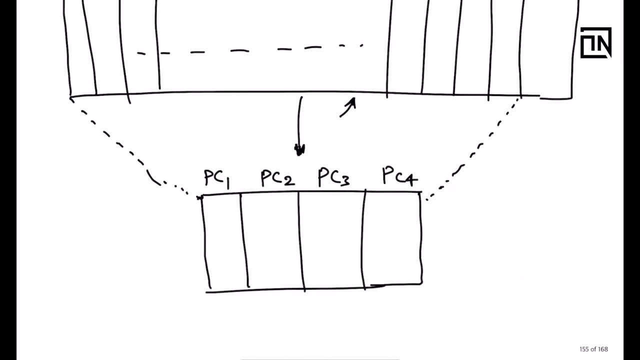 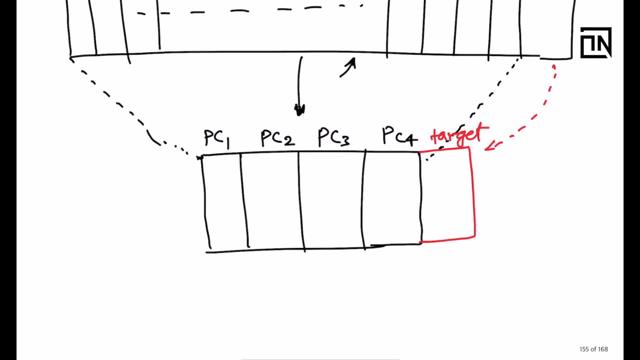 This is also something which varies from algorithm to algorithm, which we'll discuss further. Okay, So I have given this representation of 500 columns with just 400 columns. Now I can bring in the target variable, create this new data. So now this new data is a representation of the old data which was having high number. 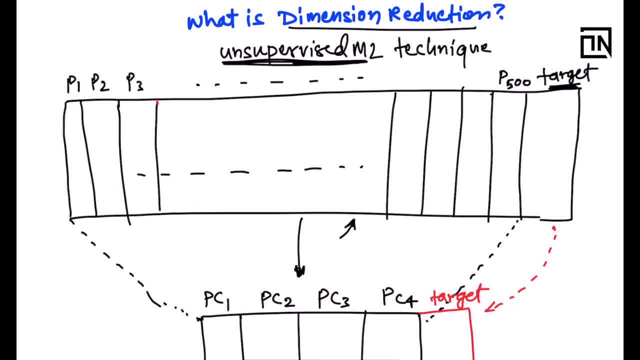 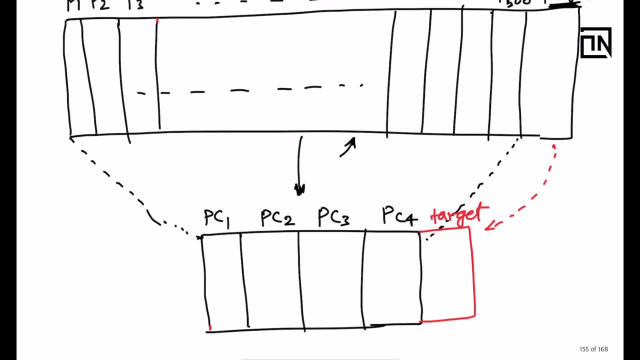 of dimensions. Dimension means what columns? So these are nothing but dimensions. Every column represent one dimensions. So if there are so many dimensions in my data because of X, Y, Z reasons, I can somehow represent it with smaller number of dimensions or smaller number of columns. 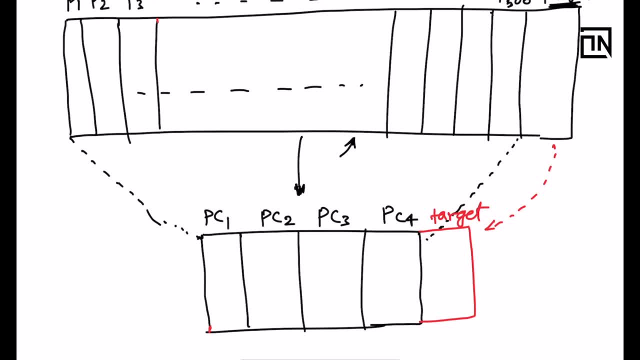 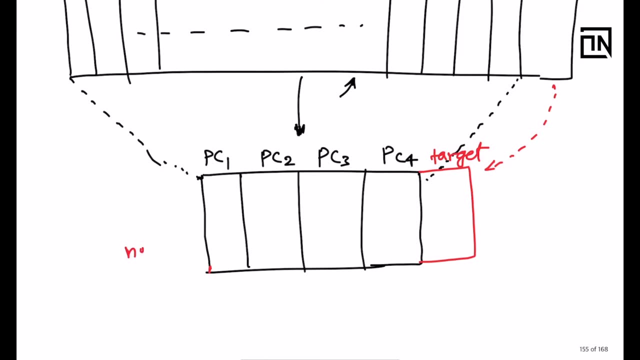 And these dimensions could sometimes be called as factors and sometimes called as principal components, etc. So different algorithms will name it differently, the way they combine it. Okay, So once you do this now, you have a new data And on this data you can fit your machine learning algorithm. 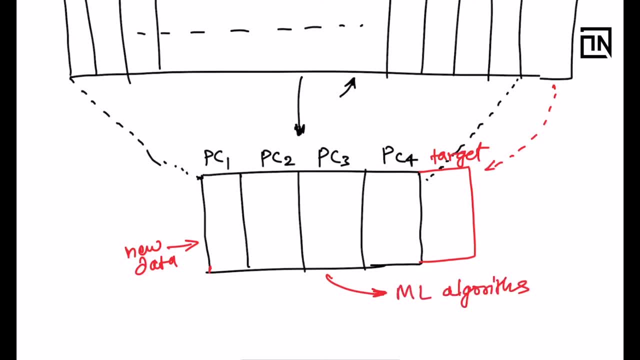 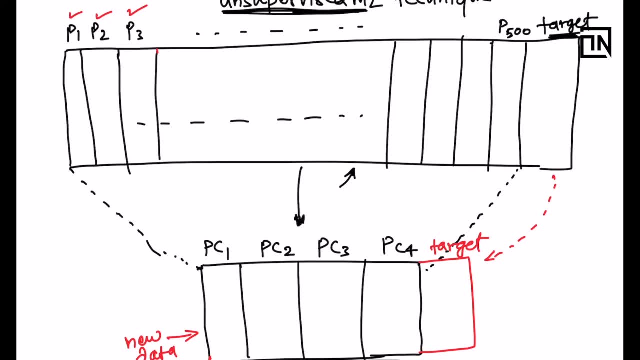 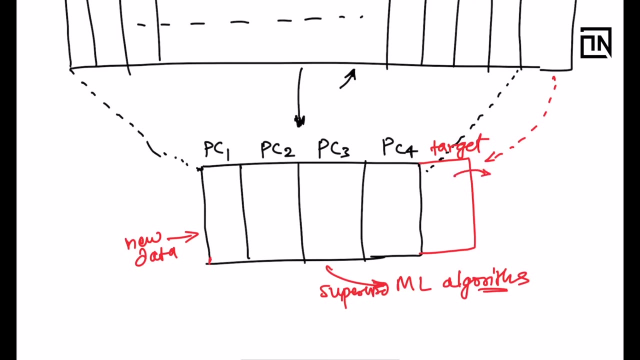 Supervised machine learning algorithm Because, let's say, the target variable is there, then definitely, either you are doing regression or you are doing classification. So, whatever is the scenario, if you are trying to predict something, which is the number, then you will fit supervised regression machine learning, or if it is a class, then supervised 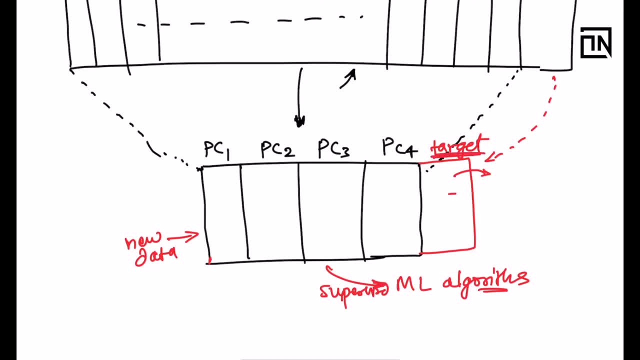 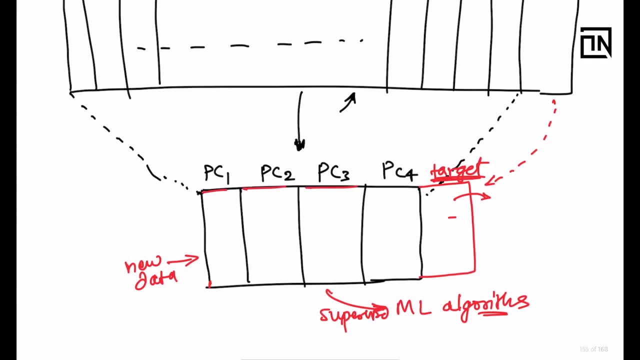 classification, machine learning, depending on the target variable. Okay, But the crux is, your predictors are now shrinked. Okay, So now you have a new data. Okay. So now you have shrinked to a smaller set of columns. Okay. 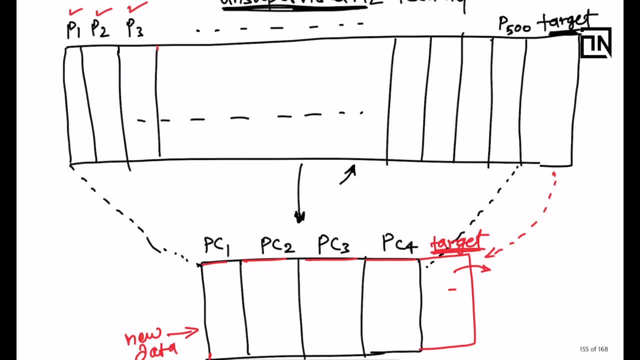 The whole journey of how these predictors are shrinked to smaller set of columns. This is something what we call as different. This is something which is very different for different algorithms. For example, in factor analysis, it will happen differently. In principal component analysis, it will happen differently. or independent component analysis. 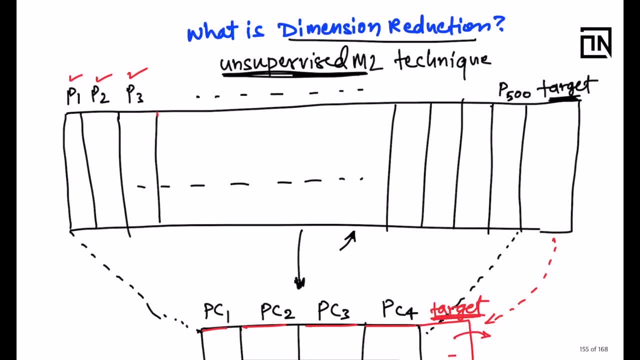 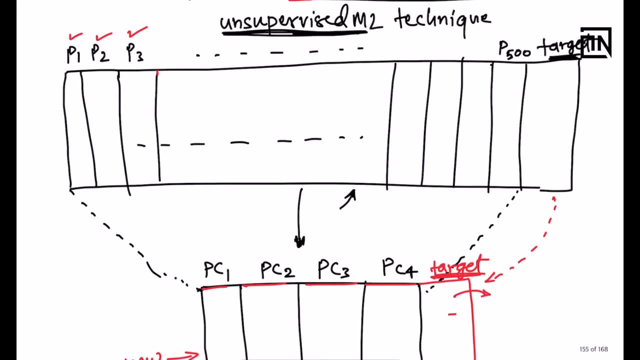 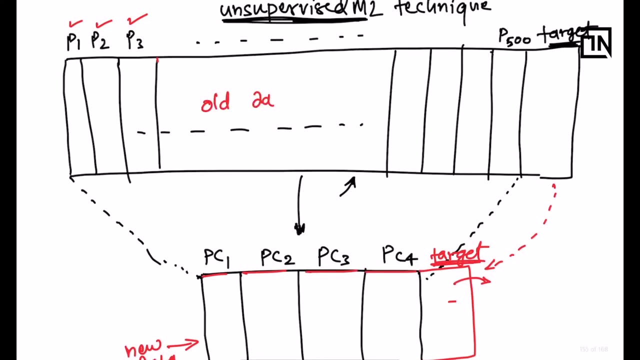 it will happen differently, So on and so forth. So what is the need for dimension reduction? Okay, So why do we require this activity to be performed? Because if you choose all the predictors, then your model training on this old data or the raw data, the model training, will be very slow. 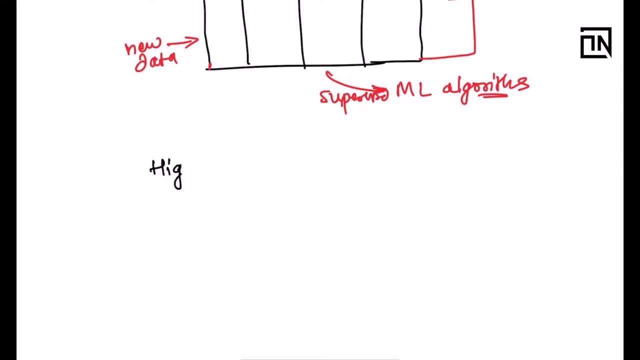 So, if your data has high number of dimensions, high dimensionality, what we call, if your data is suffering from high dimensional, high dimensionality or too many, call, too many predictors, okay. Okay, Because target variable is always one. So, if this is the issue, what it will impact on your machine learning training is first: 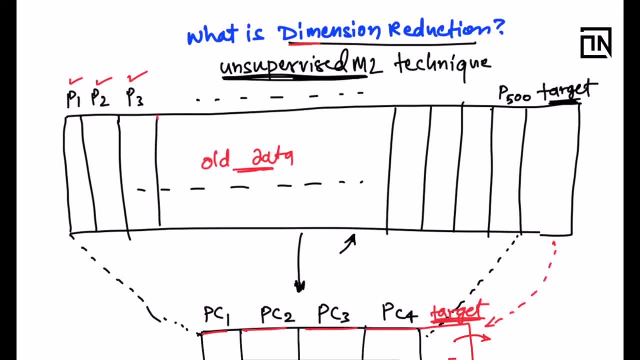 of all, it will be slow, And this is no brainer. If you have more columns in order to learn, more columns in order to find the best column out of it, or trying to find the equation of all the columns you will have, you will. 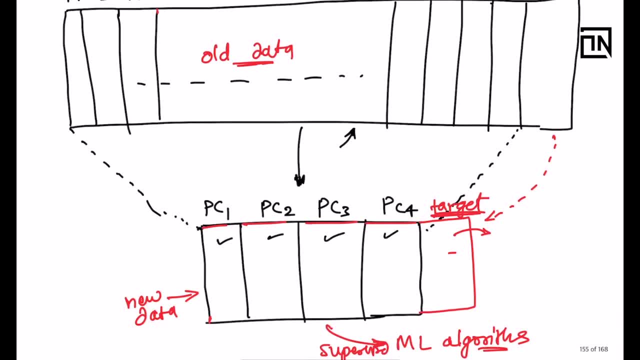 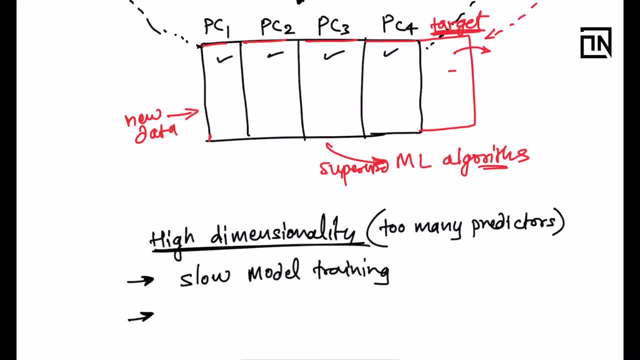 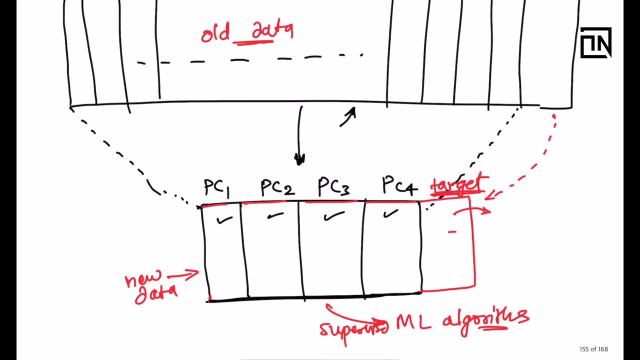 have to do more computations, And if you have less columns, then you will have to do lesser computations. Okay, So the problem will run fast. So once you convert your data into the reduced dimensions or a smaller version, or basically a compressed version of the overall data set, then you will be able to train your models. 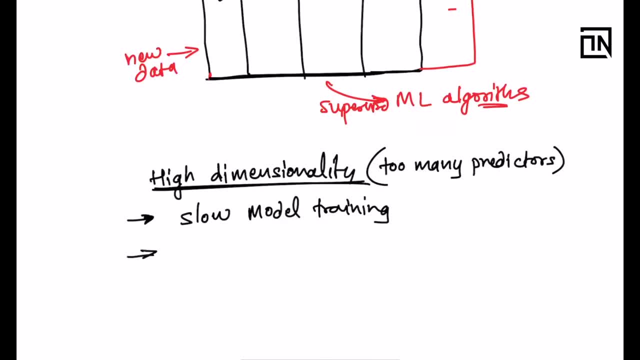 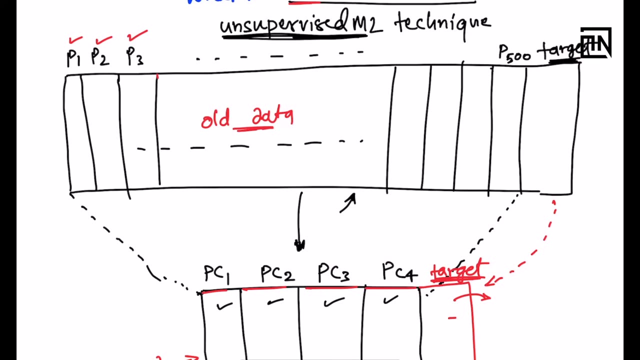 very, very fast And, due to this slow model training when your model is created, the model is also complex, which will also impact the time of predictions. So all these issues- These will come up If you have very high dimensionality in your data set and that can be resolved using dimension. 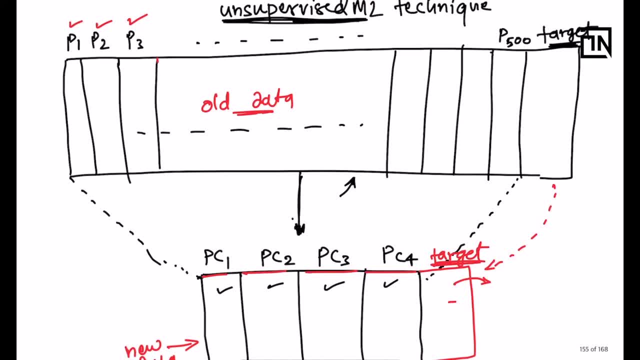 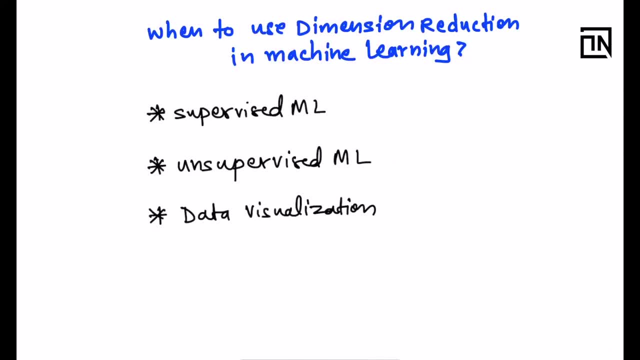 reduction, All right. So to perform this, there are many algorithms which are there, and I'll I'll quickly describe them in the upcoming section. Now let us discuss when do we use dimension reduction exactly? So we use it under supervised machine learning, under unsupervised machine learning and for 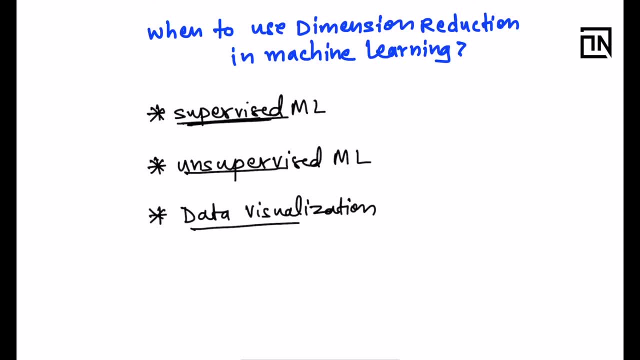 data visualization. These are the three use cases where you can Use dimension reduction. Okay, Dimension reduction, And every time, the role of dimension reduction would be to reduce the number of columns so that I can do a better job, For example, in supervised machine learning. when exactly do you employ the dimension reduction? 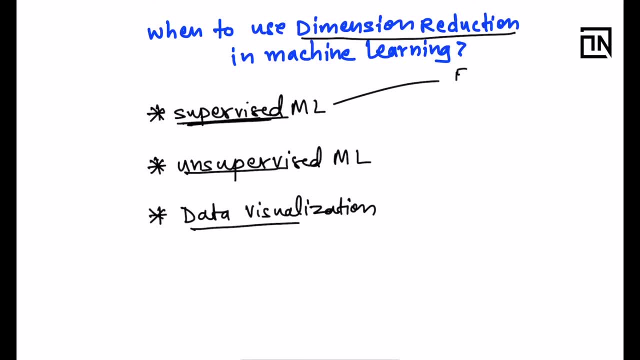 technique. So in supervised machine learning, you have done your exploratory data analysis, You have done your correlation analysis, You have selected the feature and then you have converted the columns- the categorical columns are the string columns- into number. So often, what will happen there? 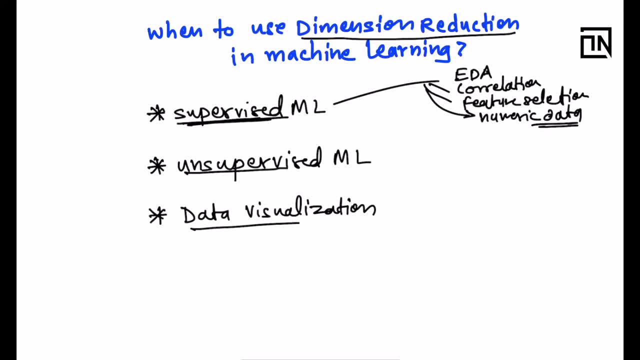 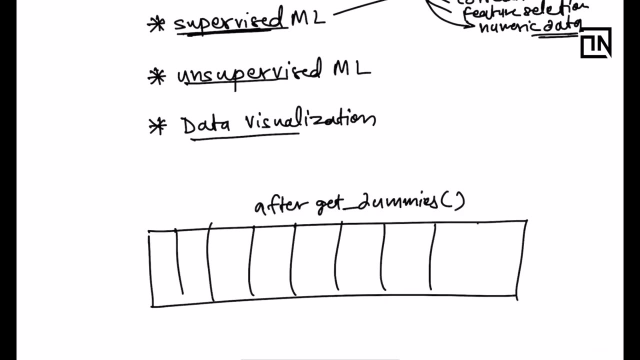 There are. there will be certain columns which have too many unique values, especially the string columns, And when you do get dummies, the number of variables will increase drastically after you do get dummies. So when each and every unique value becomes a predictor, and then you have your target. 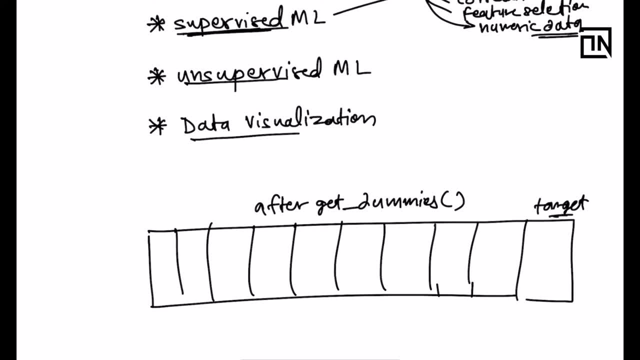 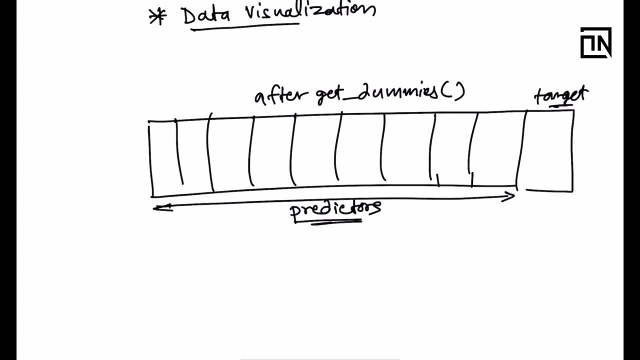 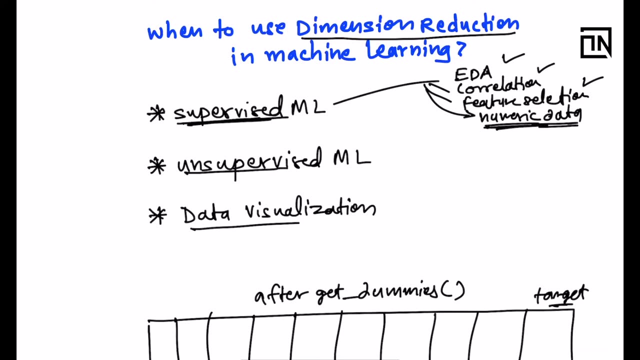 variable, So obviously it is high dimensional and the data has inflated. So in this scenario, you can choose to shrink the predictors. So when do we perform this activity? Only after all these things are done and you are at the verge of applying machine learning. 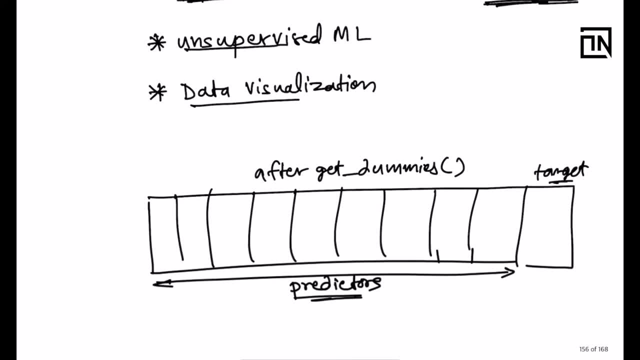 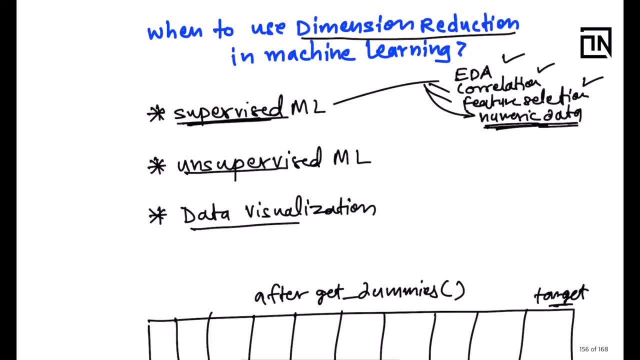 So just before that you take a call that there are too many predictors in the data, So let me try to represent them with smaller number of predictors. Okay, using dimension reduction techniques. similarly in unsupervised machine learning after you are done converting the data into numeric after this, if you feel that there. 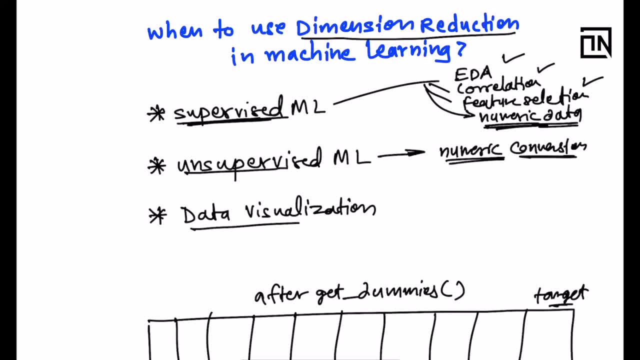 are too many columns. Yeah Yeah, This is a training process of any other unsupervised machine learning, like especially clustering, Clustering. So in clustering, before doing clustering, you can take a call that there are too many columns. So instead of doing clustering on too many columns, let me shrink this data and do clustering. 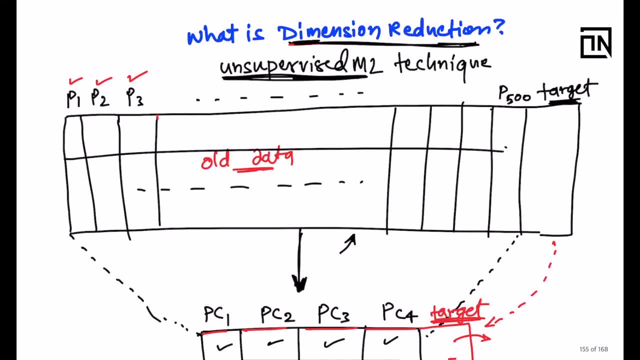 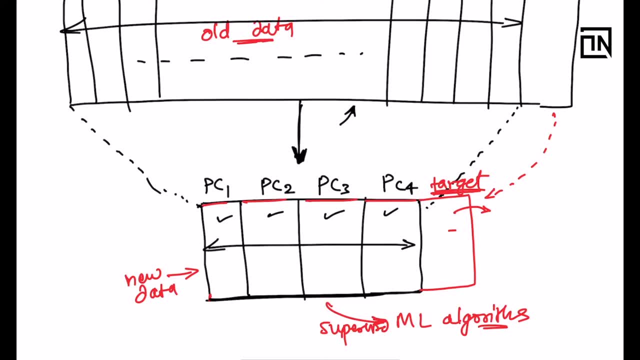 on smaller set of columns. Like, instead of doing clustering on all these variables, let me do the clustering only on these few variables. Okay, I'm just ruling out the target variable from the top. Yeah, picture right now. similarly for data visualization. so if your date, if your data has too many columns, 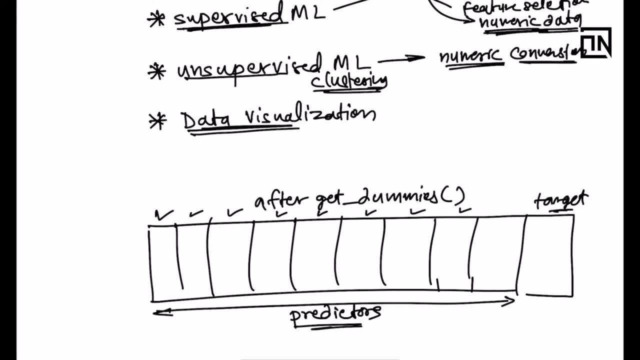 you cannot plot the n dimensional graph for all these columns, so it will be too computationally intensive as well as hectic to code. so, if you still want to, if you still want to represent the data patterns or the data variations of all these columns using smaller set of variables, so all you have to do is just choose the first two principal components of. 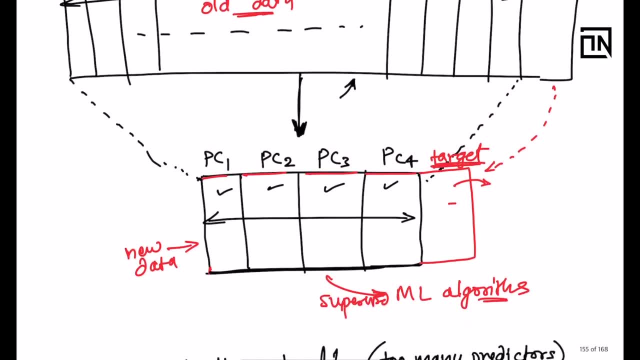 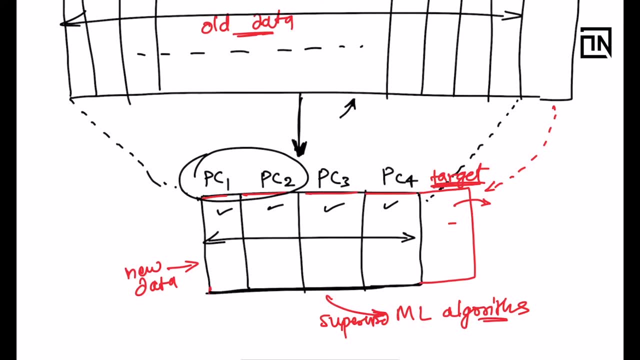 first two factors which are really important. okay, so, instead of using, let's say, 500 columns, all you have to do is just choose these two, predict these two factors which you have just generated, or these two principal components which you have generated, and then, based on this, you can create a chart. 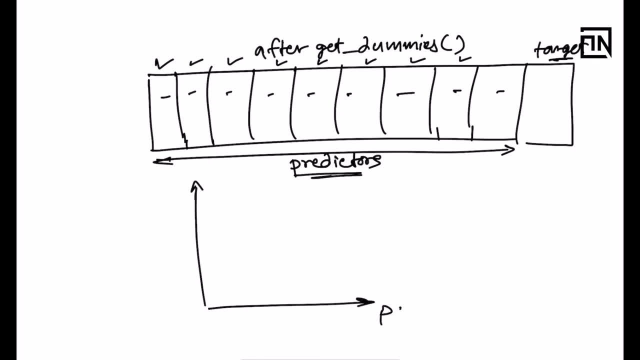 which is two dimensional, so principal component one and principal component two, let's say, for example: so data can be visualized, its grouping can be studied and clustering can be observed. okay, so when you plot a multi-dimensional data in lower dimensions or just two dimensions, you don't just 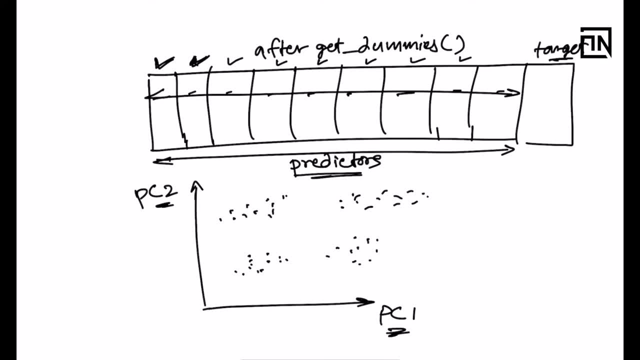 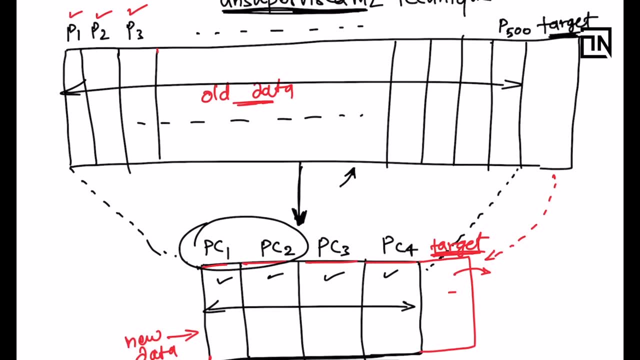 blindly choose any two columns. what you are doing is you are choosing a combination of such column because what pca, or what factor analysis, tries to do is to represent multiple such columns as a single column. okay, so there might be redundant information in multiple columns which can be clubbed together and 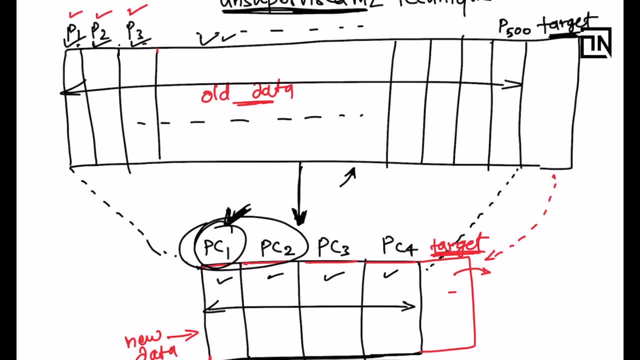 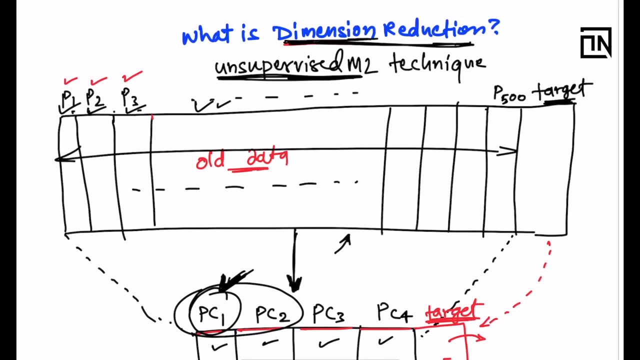 represented as one single principal component or one simple factor. okay, so combining multiple columns together, i will get my single column, or single component, or single factor. this is what dimension reduction performs for you. okay, now to perform this, what are the algorithms do we have in place? so we have algorithms like factor analysis.